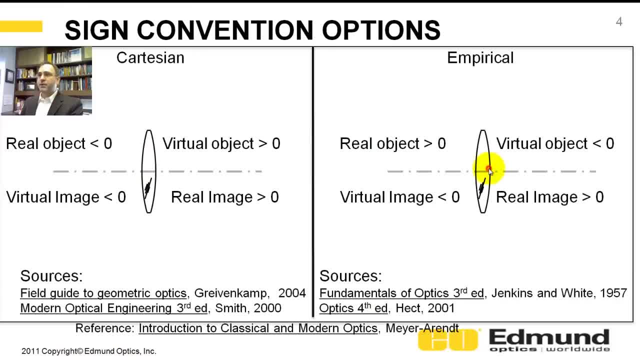 based on geometry As opposed to the empirical, where if you have a real image to the left of your lens, you're going to have a positive distance And this flips when you're doing an image to the left of the lens. It will be a virtual image. 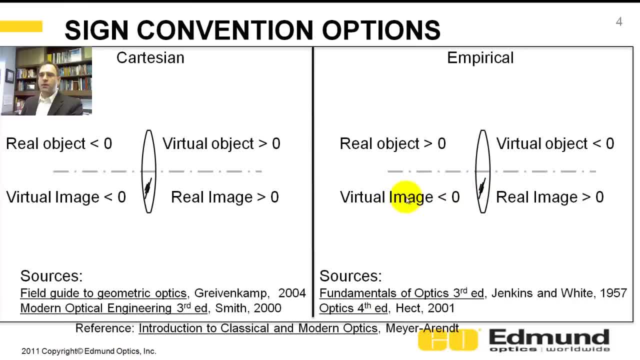 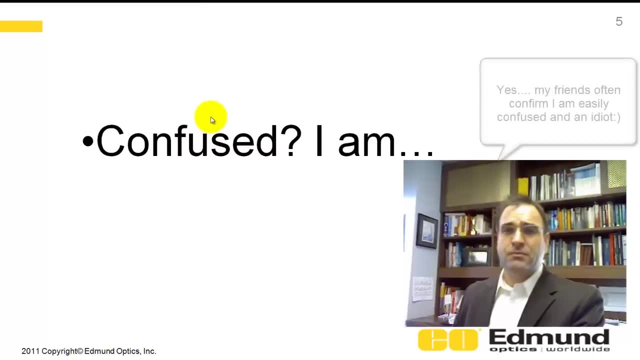 it's inside the lens, you can't physically touch it or image it onto a piece of paper. It is negative. Various sources, and I've listed them here and here. various sources use different sign conventions And I ask: are you confused? Because I am. 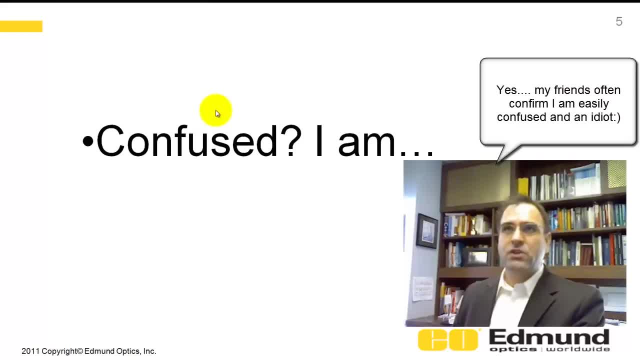 And even after getting my bachelor's in optical engineering, sign conventions really confuse me. I was forever making a mess but making mistakes, And I have another method for keeping my eyes open. I'm going to show you how to do that And I'm sure you're keeping track of sign conventions. I'll show later. 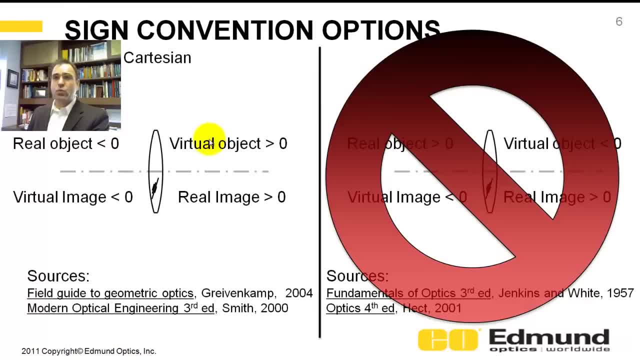 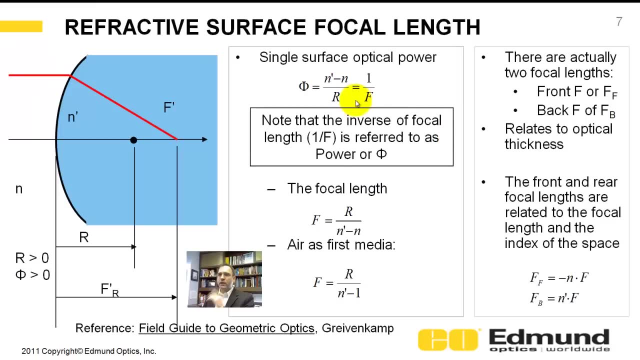 I'm not going to really try and bias you as to what sign convention to use. whether it's Cartesian or empirical, I'm going to be using Cartesian for from here on out, It's what I'm more used to, So let's talk about. 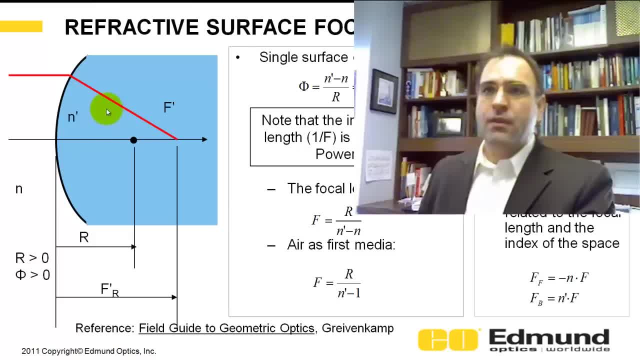 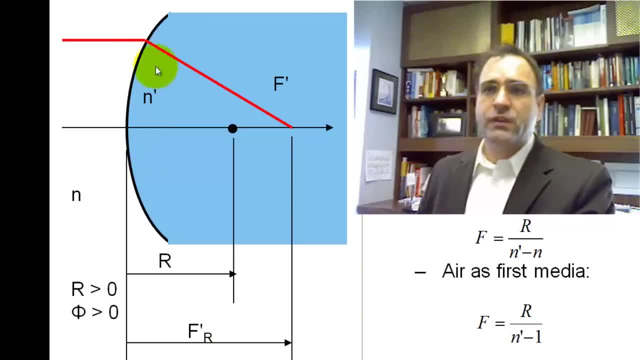 imaging through a single optical surface. So what we've got here is a piece of glass with a single spherical surface. This radius of curvature is positive if you follow the sign conventions, because the center of curvature is to the right of the surface. So what is the power of an optical surface? 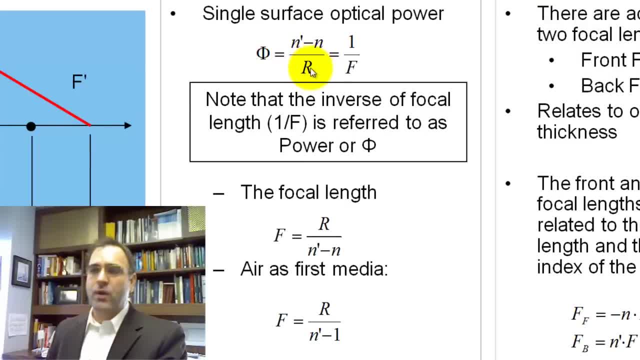 So power is the difference in index between the two media divided by the radius, And the power is actually the inverse of focal length, And we'll be talking about power a little bit later. We're going to predominantly use focal length, So the focal length is really the. 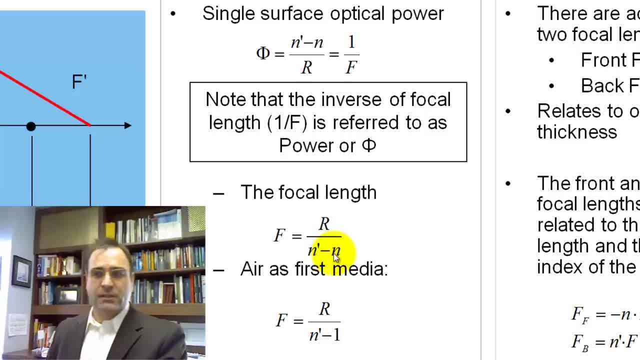 radius of curvature divided by the differences in index of refraction. If your first media, this media here, is in air, your focal length is simply your radius of curvature divided by your index minus one. There's actually two focal lengths: There's a front focal length here and a 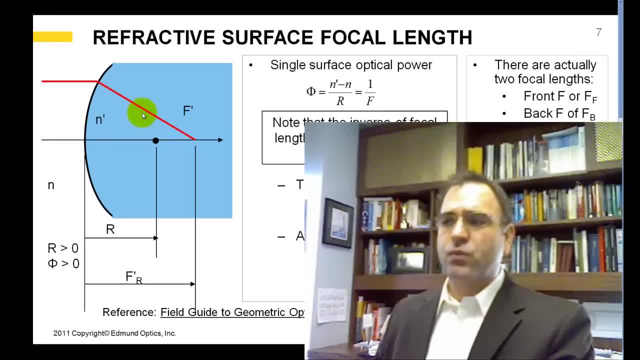 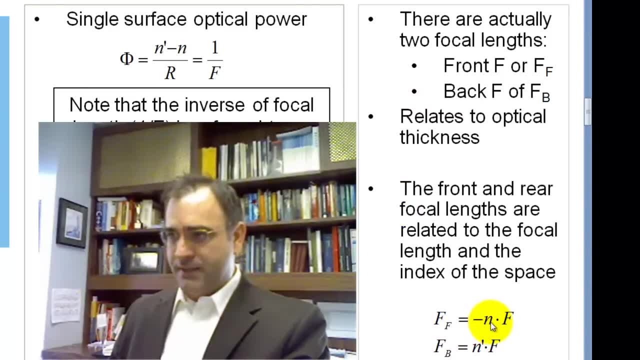 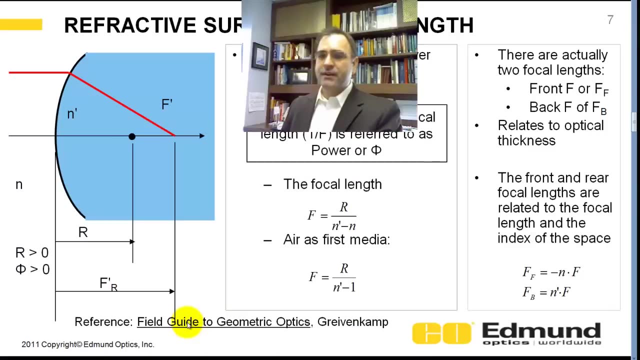 back focal length here, And those focal lengths relate to optical thicknesses. I won't go into detail there, but the equations for the front focal length are minus n times f And the back focal length is n prime times f. The reference here is this field guide to geometric optics by John Grevenkamp. 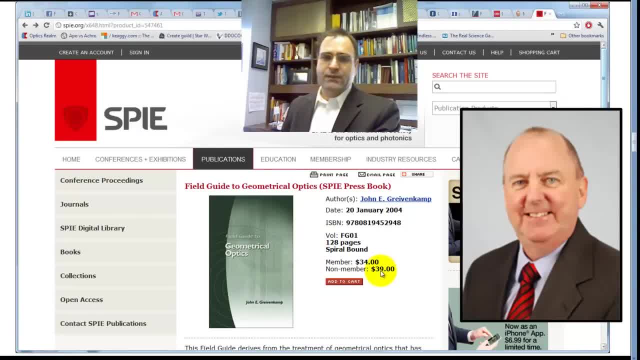 It's a cheap, cool little book. It's forty bucks for a non-member from SPIE. It's chock full of great knowledge and great equations and John does a great job of teaching it, And I took his graduate and undergraduate classes- and, yes, I'm biased for him- and 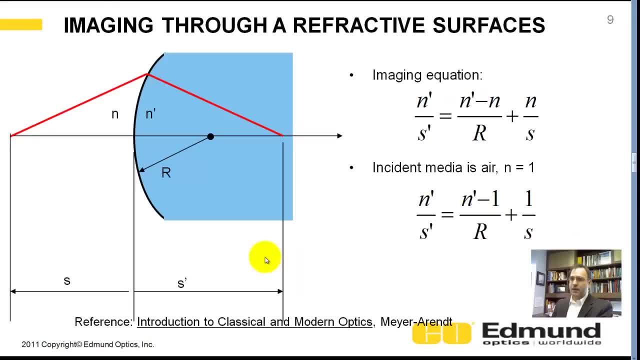 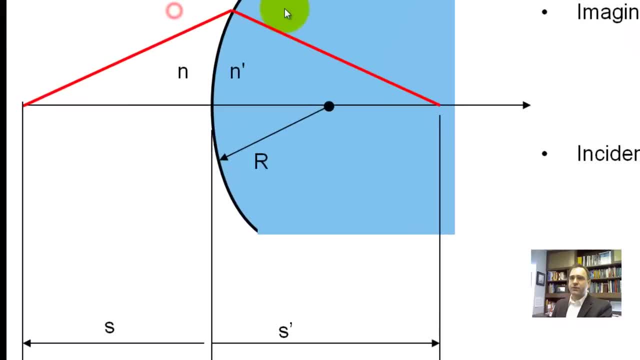 I'd like to see him profit, but the book is really good. It's really worth its money. Let's talk about imaging through a refractive surface. Now, because you've got two different index of refractions, you can use this imaging equation here And again, this uses the Cartesian. 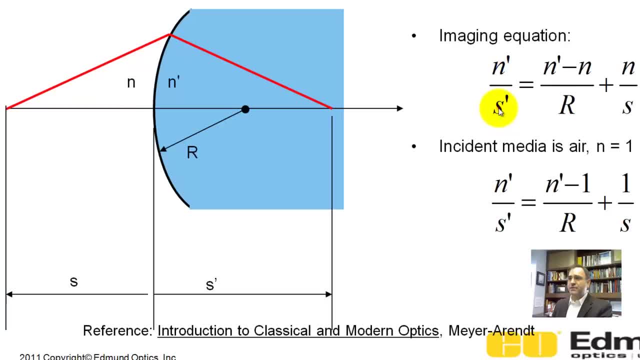 coordinate system: N prime divided by s prime. This s prime is your image distance here Is equal to the difference in the index divided by radius plus your incident media divided by your object distance. If you're in air, the equation simplifies to two. 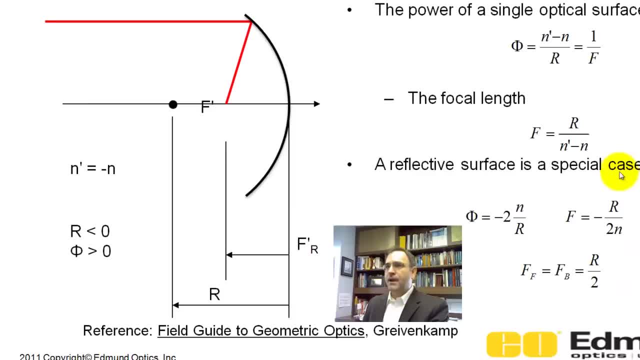 Etc. You could say it's a próxima equation if you use Reading 아무다르�지 rgrorg For a reflective surface. I'm not going to go into much detail Again. I'll reference you to Green in Camps book. 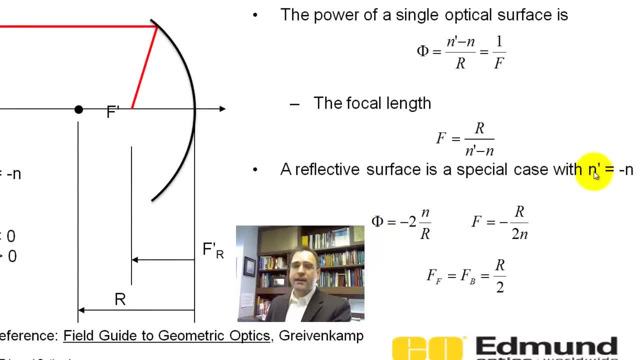 I just want to point out that for a reflective surface this is a special case where your secondary medium is actually the negative of a, your incident medium. So n prime here equals negative n, And the consequences of that was your focal length is your. 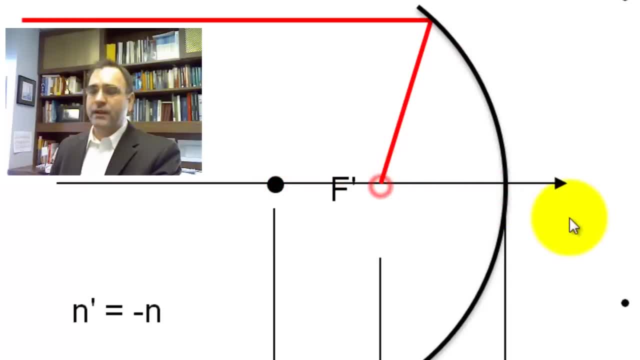 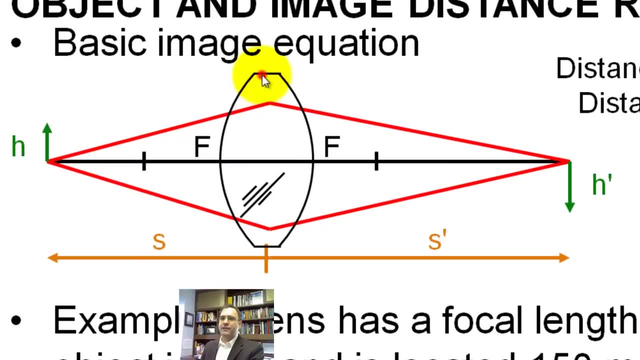 center of curvature. so from here to here is your radius. your focal length is halfway in between there. Let's talk about imaging through a lens. Now I've shown a thick lens here. This equation works for a thin lens, meaning infinitesimally small. It's a first. 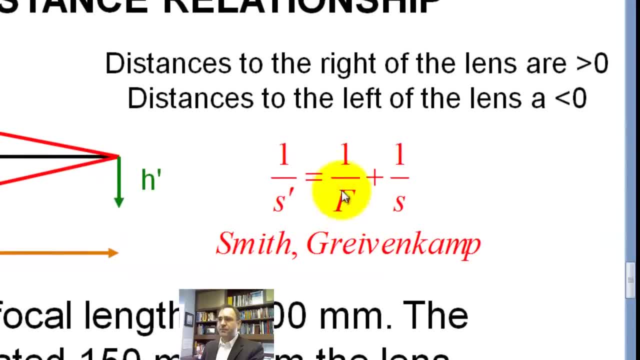 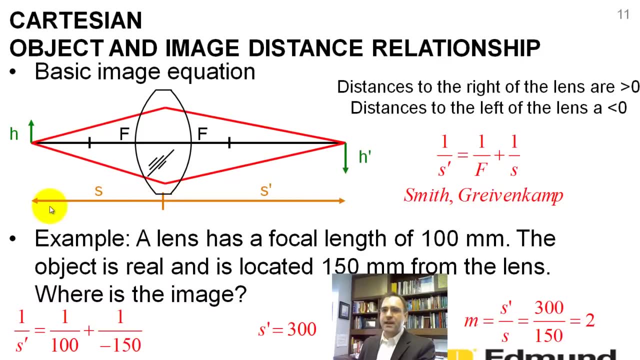 order equation. This is using the Cartesian coordinate system. The equation is 1 over s. prime equals 1 over f plus 1 over s. Again, this is a Warren Smith or John Grievenkamp nomenclature, And if you have a real image, like is here, your s is negative. So let's. 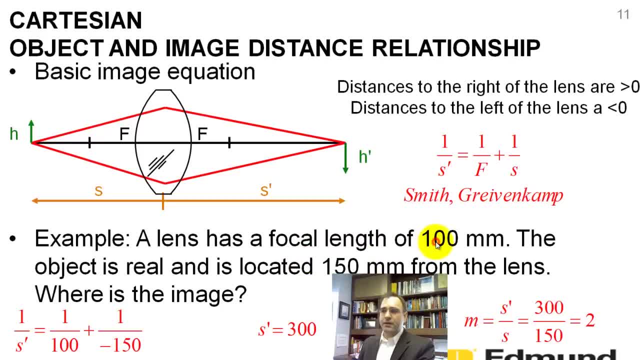 give an example. Lens has a focal length of 100 millimeters and the object is real and located 150 millimeters from the lens. Where is the image? Well, you plug and chug. you've got to know that this 150 is really negative. You plug and chug into your equation. you 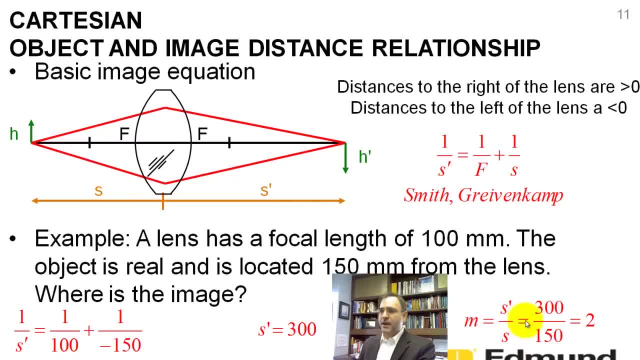 get s prime to be 300. And oh, by the way, the magnification is roughly 2.. I'm waving sign conventions here As opposed to the empirical equation. there's actually a negative sign here between your focal length term and your object distance term, And I'm forever messing this up, Hopefully after doing. 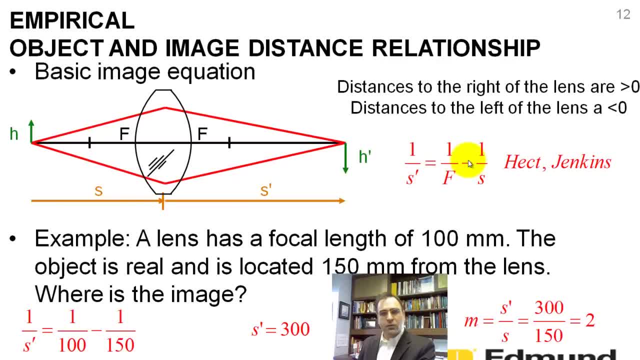 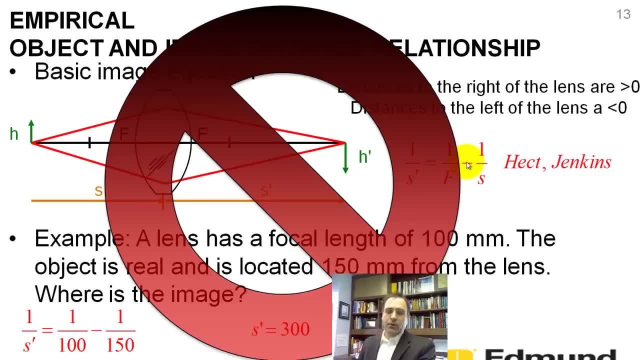 this PowerPoint presentation, I'll be more apt to remember this Again. I'm not going to bias you, but I don't like this method, so I'm going to put a Buster Sign through it. We talked about magnification. Magnification's a parameter for understanding. 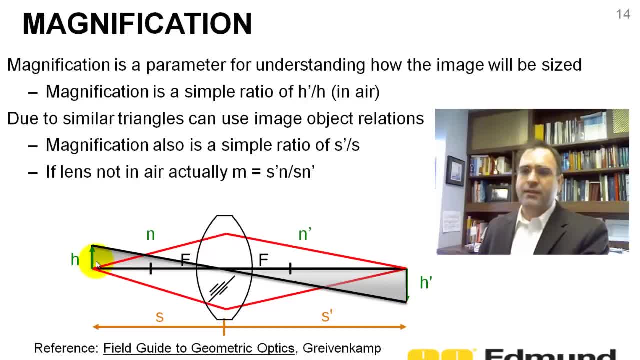 how the image size or image height is a function of the object height And for a lens in air, it's simply a ratio of h prime over h. Now, because of similar triangles, this h and this s versus this h prime and this s prime, magnification is also a simple ratio. of your image distance divided by your object height, And once you're able to do this, you'll be able to get at this point. You'll have a very distinct and very clear picture, And it's a very small percentage of your image size, And I'm going to give you a little bit. 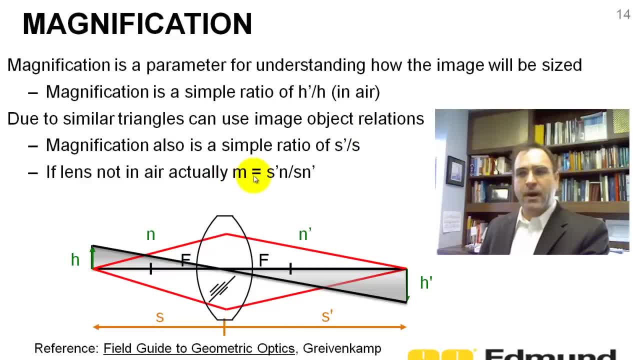 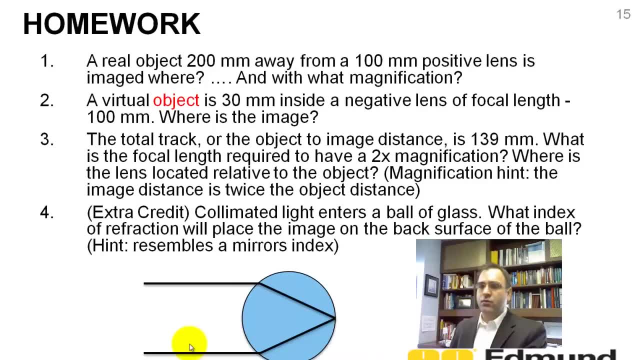 object distance. If your lens isn't in air, you've got to worry about reduced thicknesses. It's S prime N divided by S N prime. Again, I reference John's book, great book. Here's some homework, very simple homework, very straightforward, except this last one. This 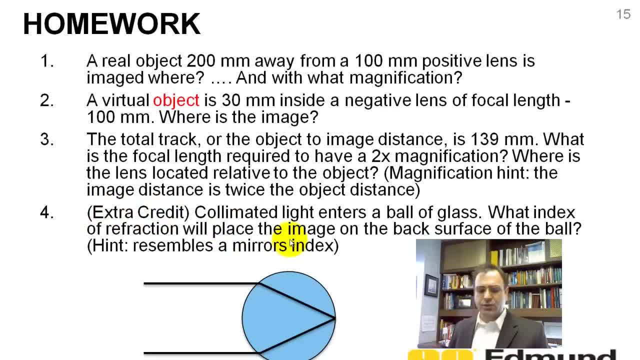 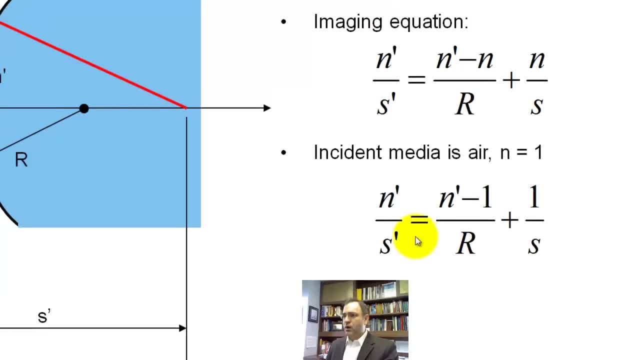 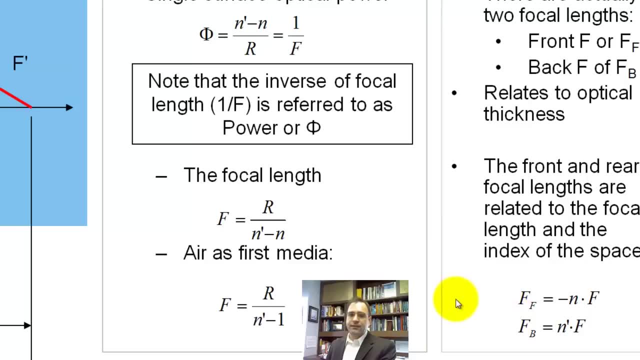 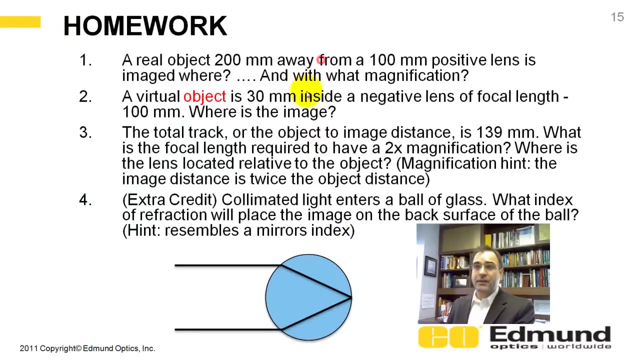 last one extra credit here. I would encourage you to use this equation here. This equation will work out. You can do the last homework with these equations, but it gets confusing And again, I believe that doing some of these, you're going to be a little bit confused because 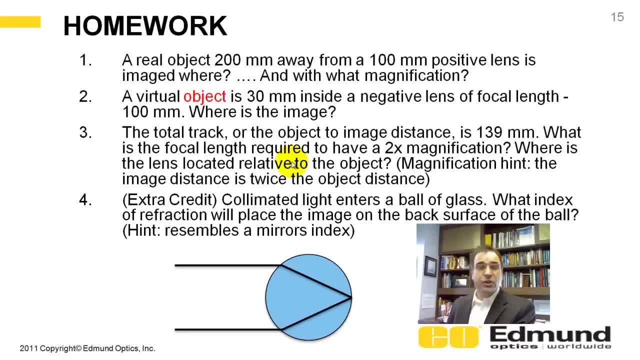 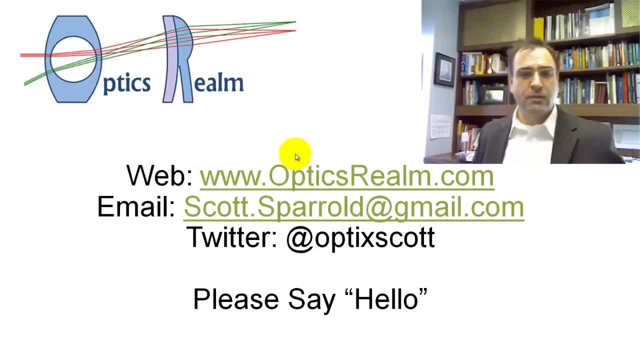 sign convention, and that's probably my fault because I showed you both, but I want to show you that sign convention can be confusing. Next time I'll talk about an imaging nomograph that helps me visualize how lenses and mirrors work. Thank you for paying attention. If you have feedback, please visit my website at opticsrealmcom. 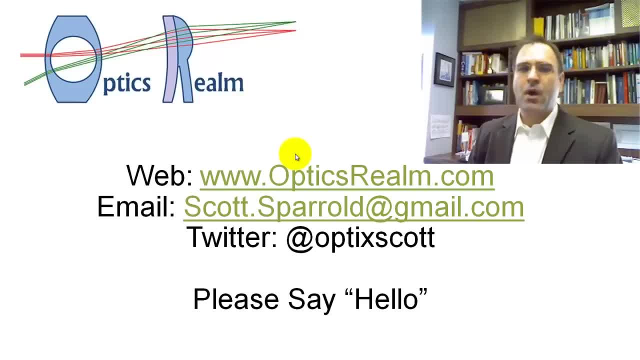 You can get me on email- scottsperlgmailcom- or on Twitter. Yes, when I set up my Twitter account, I did not know how to spell optics. Thank you and stay tuned.